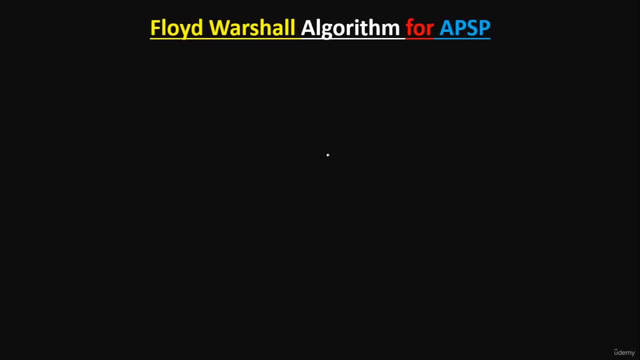 hey, what's up guys? welcome back to this video. in this video, we're going to talk about Floyd or shell algorithm. now let's talk about how Floyd or shell algorithm works for all peer. shortest path problem. let's add him. we're given this graph. this is our graph data structure. this graph is a weighted directed graph. this: 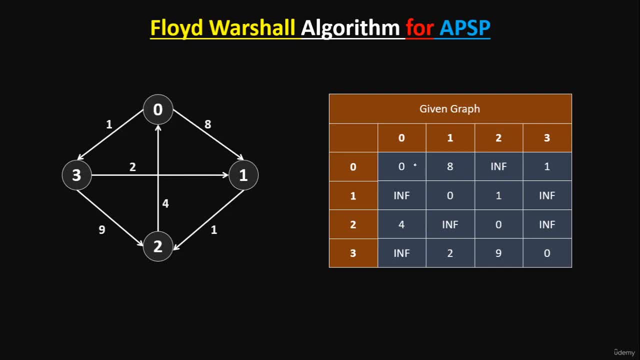 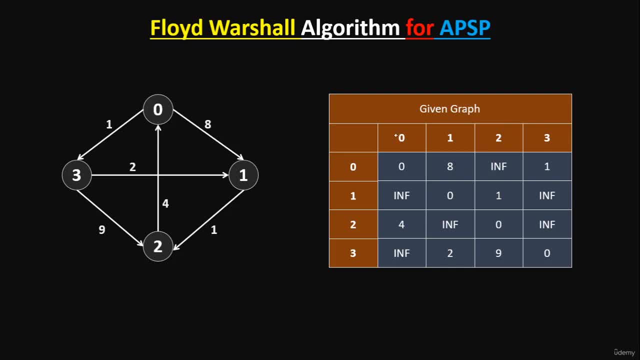 node is 0, then the distance in between 0 and 0 is 0, because we have here no self loop: 0, 1 4 0, 1. we have 8 4 0, 2. we have infinity, because we do not have any directed edge that goes from 0 to 2. 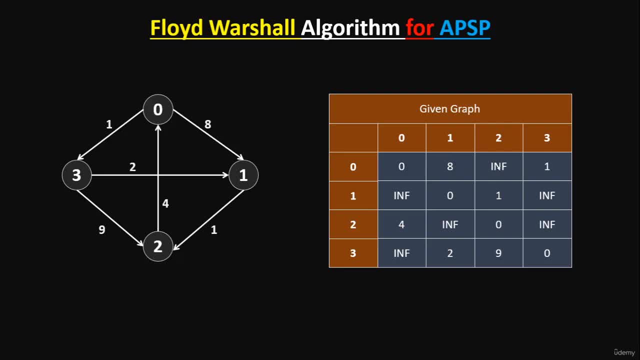 that's why we have here infinity. we're representing infinity as maximum integer we can store in 32 bits. here we have 1, 0 to 3. we have that weight 1. then from 1 to 0, infinity, because we do not have an edge. from 1 to 0, there is no. 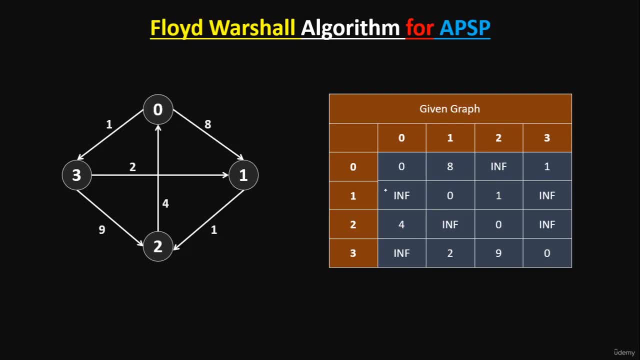 outgoing edge from 1 to 0. that's what we have here. infinity and so on. hope you have understood the representation of this graph data structure using this adjacency matrix. now let's talk about how Floyd or shell algorithm works. Floyd or shell algorithms uses the concept of dynamic programming. now let's review the 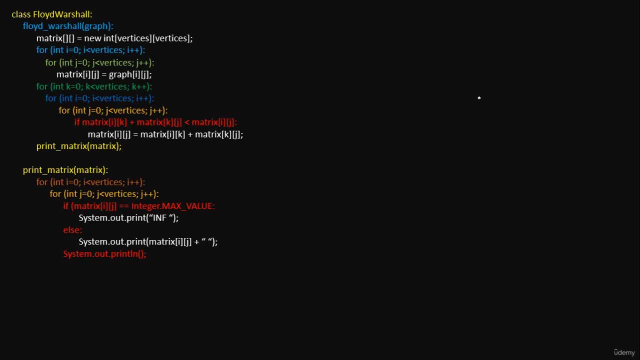 algorithm. then we will see how this algorithm actually works. we'll go through a line by line and we'll explain every bit of information that we need to understand Floyd or shell algorithm. we have here this clutch, Floyd or shell. inside here we have two method: Floyd or shell and print matrix. 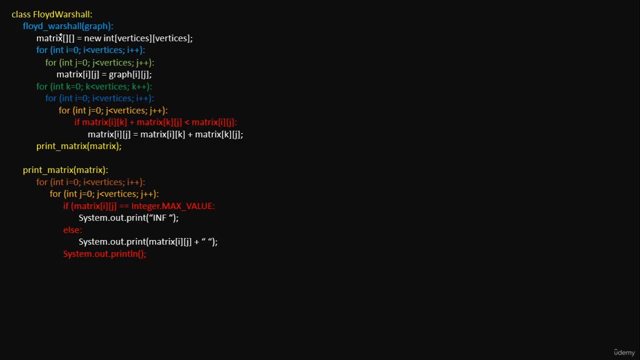 this algorithm, this function- Floyd, underscore or shell- takes the given graph as input, the given graph as a adjacency matrix. here we're creating matrix new and vertices, vertices. then we're running this nested for loop to copy and the value from our graph data structure to this new adjacency matrix. then we're 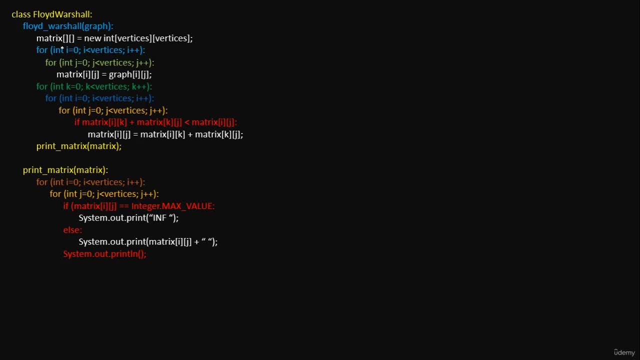 running this nested for loop to copy the value to matrix. we're running your algorithm- here we have three nested for loop- and inside here we're checking if I K plus matrix K J is less than matrix I J, then we're applying this formula and at the end we're printing the matrix. here we have the code for printing the matrix. 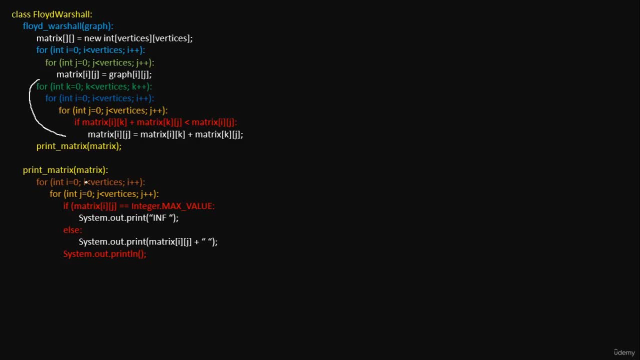 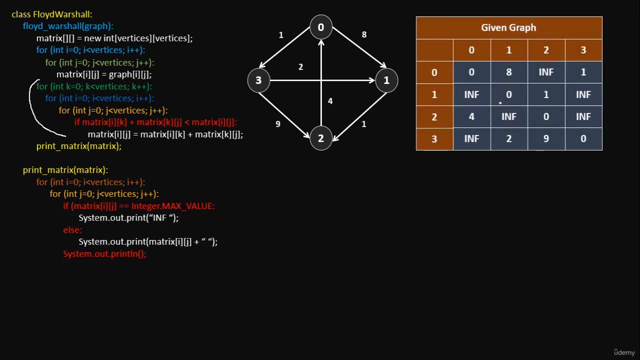 now let's see how this algorithm actually works. a jumpy confused about it. we're going to explain every single information of this algorithm. let's assume we're given this graph and this graph is represented using an adjacency matrix. this is the adjacency matrix. let's copy this graph to this metric. so 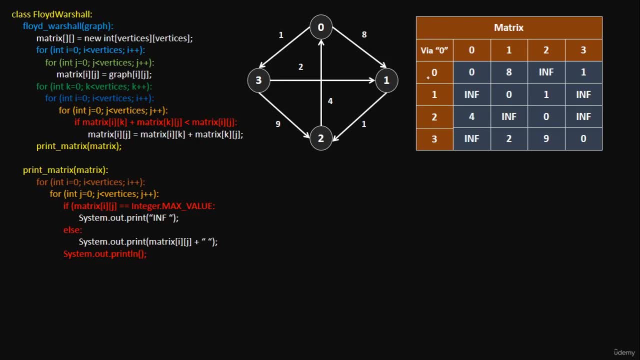 if we copy, we get this matrix. now, first thing, what we're going to do, we're going to find a path that goes via the vertex zero. So here, what we're going to do, we're going to find it. all pairs, okay, Every pair, first 030102, then 121013, and so on. we're going to generate every. 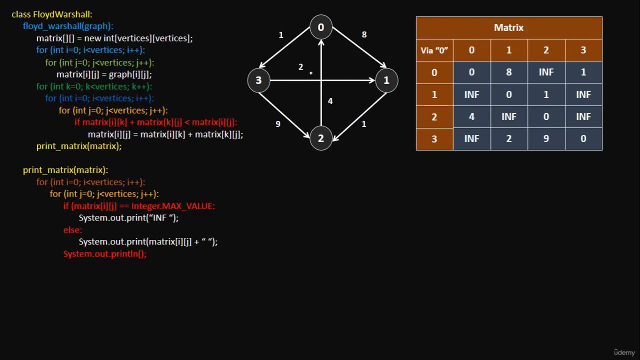 single pair from this graph And we will find out the minimum distance between two pairs that goes via the vertex zero. After finding out all possible peers and calculating minimum distance, we will we will see the minimum distance for the peer that goes by one, two and three. Now let's find. 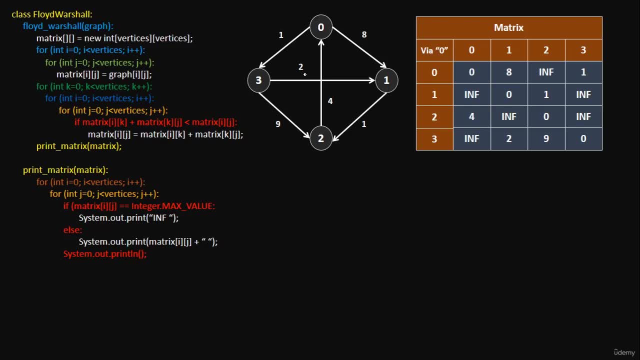 out the minimum distance between two pairs. So here we're going to generate every single pair, the minimum distance for all peers that goes via the vertex zero. Let's see how to find out that. Here we have the iteration okay, k equals to zero And here we have ig. we have a, two nested 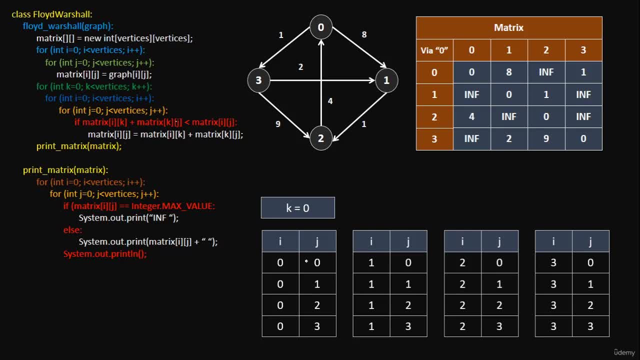 for loop inside. So this two nested for loop will execute 000102031011, and so on until three. three. so let's see how to find out minimum distance path that goes via zero. here zero means k, so we can. 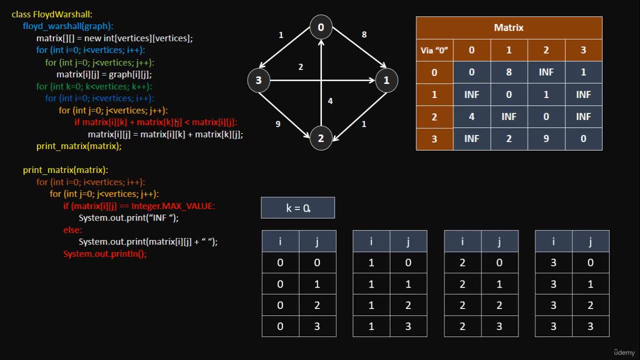 say, the minimum distance path that goes via zero- First we have zero. zero, Now we're going to check, does disappear- goes via the V attack: Zero. here we have zero and zero And we see this value is zero. Also, here we're going to apply this principle to some sampling Madonna. Huge Business, So siellä. electric is called Expansive Source Poem, Also a wedding single Assassin. Does a�be awesome, Right, we're going to check. does this? prior goes via that for x: zero. here we have zero and zero And we see this value is zero Also here. 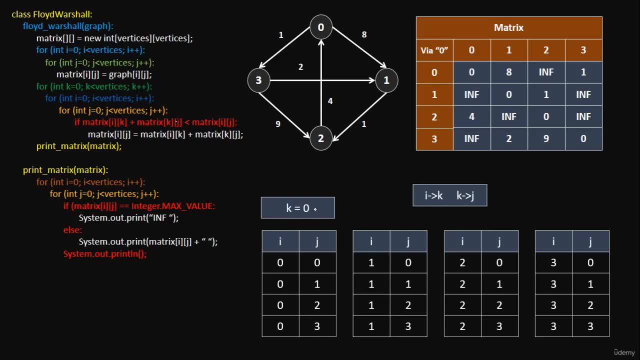 we're going to apply this formula: the distance from 0 to 0, that means from i to k and from k to j, from 0 to 0 and 0 to 0. we see, for 0 to 0 and 0 to 0 we have value 0, the path from 0 to 0 and from. 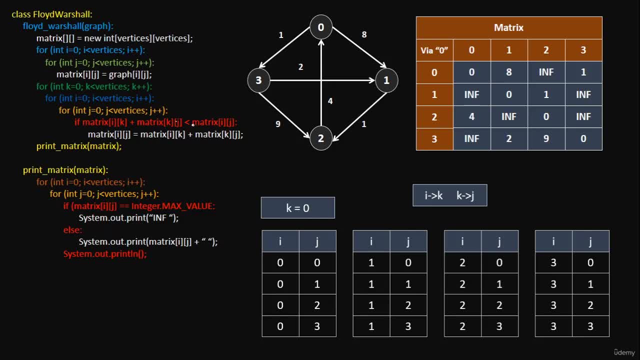 0 to 0 is 0 plus 0, that is 0, and we see that the current value here, 0- 0, is not less than 0, so this value is evaluated false, so we'll not update this value. okay, now let's move to the next pair: 0- 1. 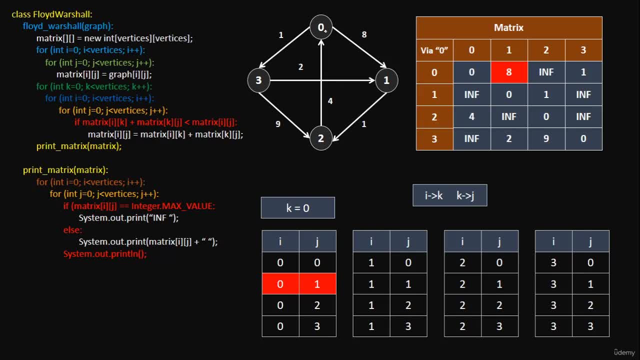 does this pair go through the vertex 0? we're going to find out the distance from 0 to 0, that is 0, and from 0 to 1, and that is 8. 0 plus 8 is 8. it is not less than 8, so we'll not update. 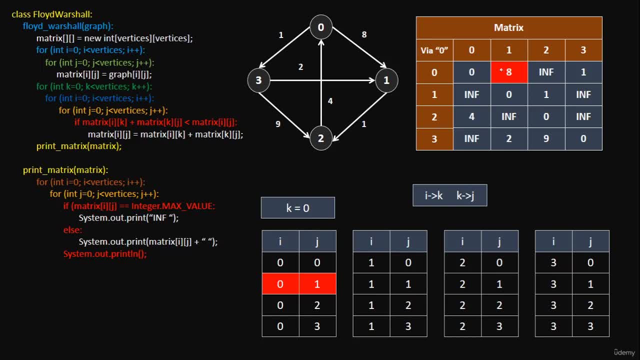 this current value. here we're generating all possible pair that go through k, so we'll have minimum distance. okay, this is kind of a dynamic programming, because we're using the previously calculated result to find out our current result. now for 0 2 0- 2 0 0 and 0 2 2 0- 2 is infinity, infinity plus. 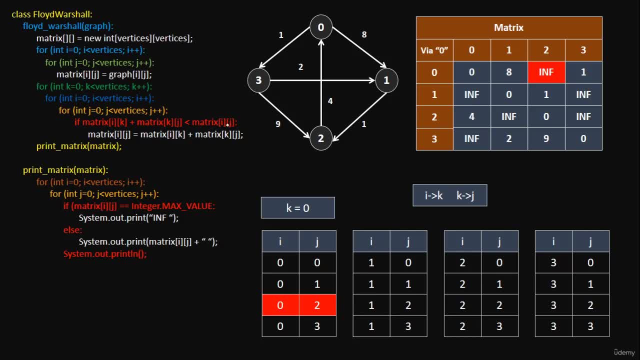 zero is infinity. infinity is not less than infinity, so we'll skip this value. will not update this value. let's move forward now. here we have this current value 1, and we have pair 0, 3, 0 and a 3. this is 0 and 0. so from 0 to 0, the value is 0 and from 0 to 3 the value is 1, 1 plus 0 is. 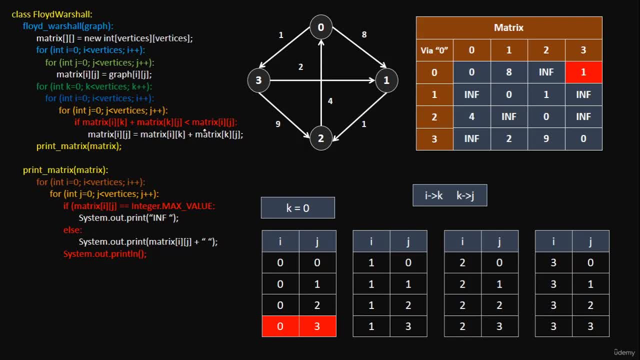 1, so 1 is not greater than 1. so all update this value. let's move forward. now we have this pair: 1, 0 for 1 0, 1 2 0. that means from i to k, 1 to 0. we see that there is no direct path. the value is infinity, infinity plus 0 to 0: infinity. 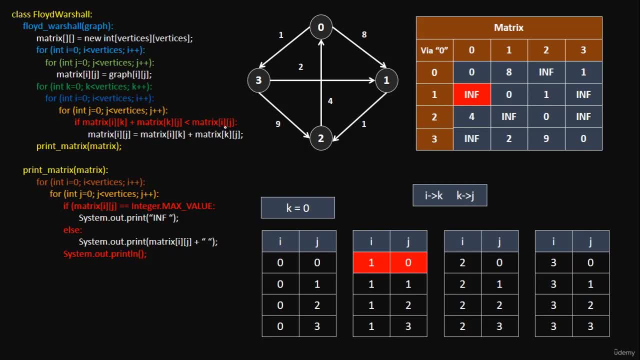 plus 0 is not less than infinity. so let's move forward here we see that we have the value 0 and we have here to pair 1 and 1. for 1 and 1 we have the value 0 1, 0. infinity 0, 1, 8. infinity plus 8 is: 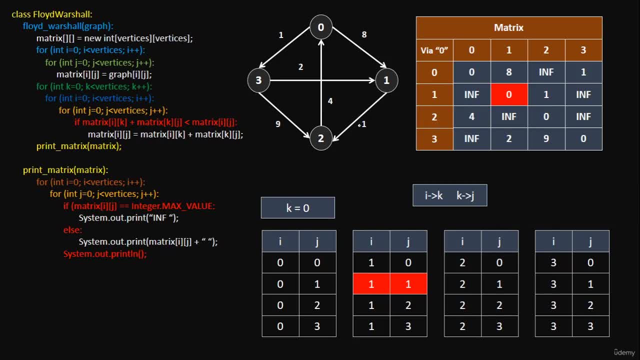 infinity infinity is not less than 0, so we will not update this current value. let's move forward. now we have this pair: 1, 2 for 1: 2. we see that from 1 to 0, from 1 to 0, values infinity, infinity plus. 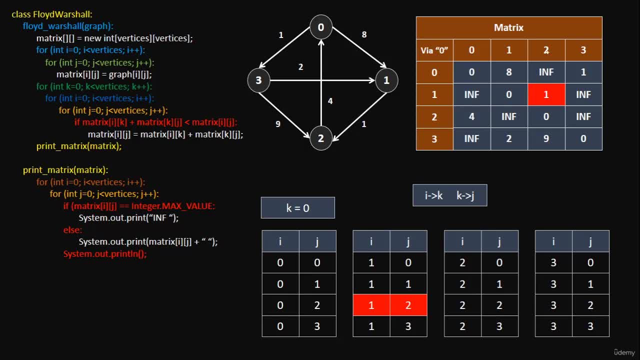 0 to 2. 0 to 2. we see that the value is infinity. we see that we cannot find out shortest path for this pair that go through 0, so we'll not update this value. let's move forward now. we have here infinity and we have 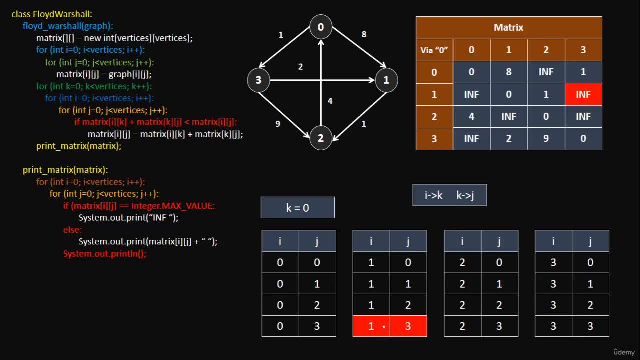 this: two vertex, one and a three. from one to zero, from one to zero, value is infinity. so if we find it infinity, nothing need to be done here. let's move forward. here we see that two, zero to zero, we see it go through zero. so two to zero is four and zero to zero is zero. four plus zero is 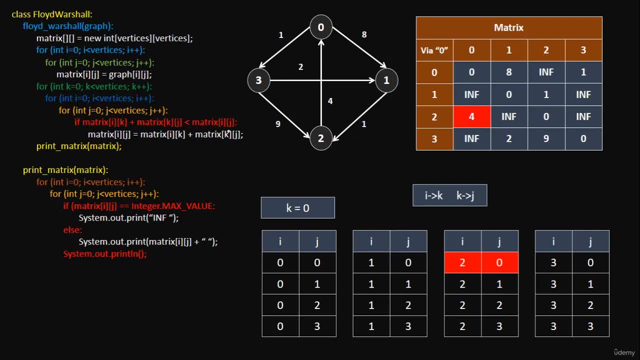 four. and we see, four is not greater than four. so let's move forward. now we have here infinity. now we have this pair to one. here we can consider i as source and j as destination. can we go from this source to destination via k? let's see two to zero. two to zero is four, four plus zero to one. zero to one is eight, four plus. 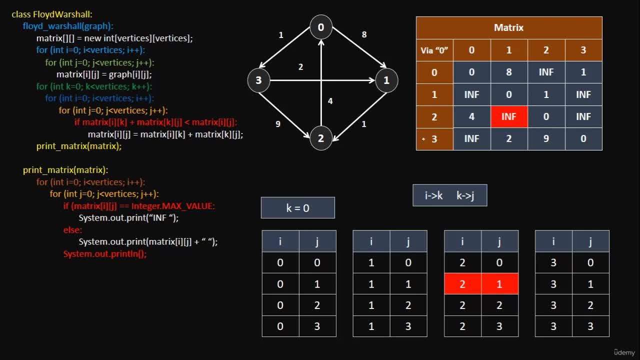 eight is twelve, we can right. so twelve is less than infinity. so let's update this value here with twelve. now let's move forward. we see we have here two. two now for two, two. we have no loop here to visit the vertex two. from the vertex two, the minimum distance is 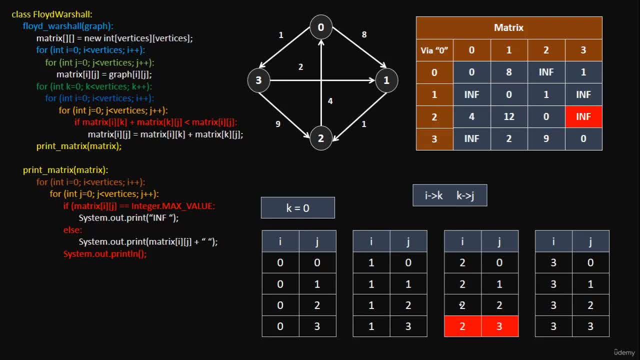 zero, because it's refers the same node. now two, three, from two to zero, we see four plus zero to three, zero to three, that is one. so we get here: four plus one, that is five. let's update this value with five. so here we see: two is source and three is destination. two is source, three is destination. 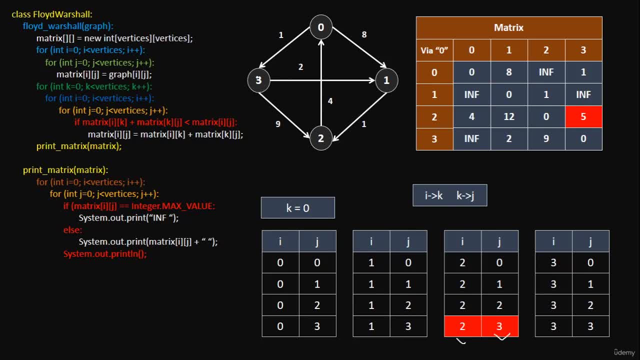 and we can visit this destination from this source, true, via the vertex zero. so we find out a value here now. let's move forward now we have three zero for three zero. now, from three to zero is infinity, so nothing need to be done here. let's move forward now. three, two zero. three, two zero is infinity, nothing need to be done. 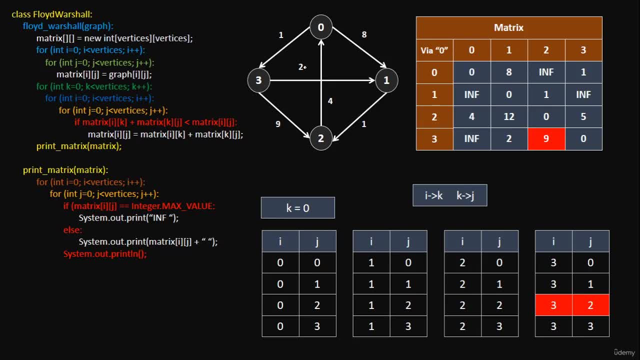 here: three, two zero, three two zero is infinity. we have no outgoing. direct is here now, from three to zero, it's again infinity. so nothing need to be done here. so we have processed all pair that can go via the path zero. so we have processed all pair in this graph that might. 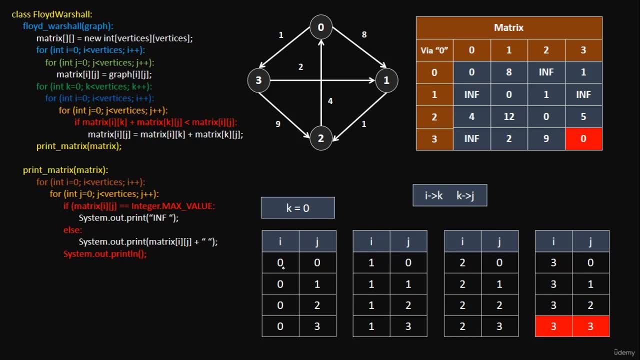 visit the destination from the source. here j is destination, i is source. so in this graph we saw that. in this graph we saw that we can move from source to destination except zero to two, one to zero, one to three and three to zero. now let's choose the vertex one here. now we're going to find out. 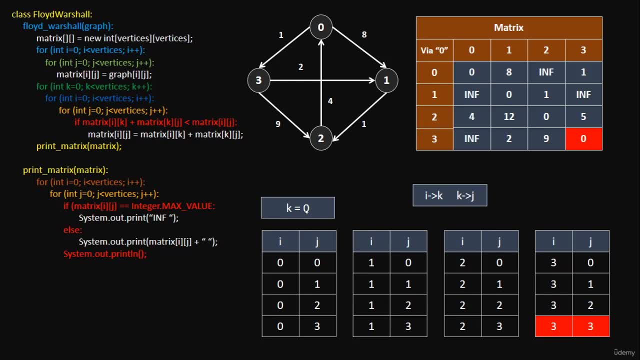 all pair that might go via the path one. now we have k equals to one. first we have zero, zero for zero. zero zero to one is eight and one to zero, one to zero is infinity. so let's move forward here, because infinity plus eight is not less than zero. now we have here eight. we have to visit the 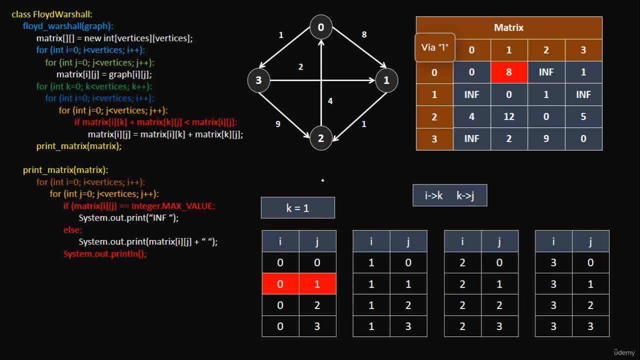 vertex, one destination from zero. so here zero to one is eight and one to one is zero. so we see that we have here eight, so we'll not change this value. let's move forward. zero to one is eight and one to two is infinity, so we'll not change this, because infinity is not less than infinity plus eight. 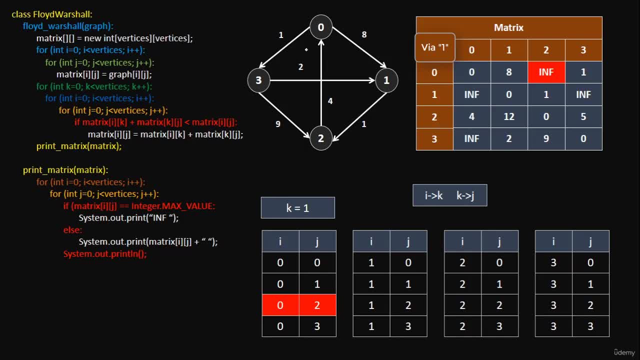 let's move. now we have zero two. from zero to two, we have to visit this. eight plus one is nine. nine is less than infinity, so let's update this value with a nine now. now we have zero three. so here we see that we cannot go from zero to three via one, so we'll not. 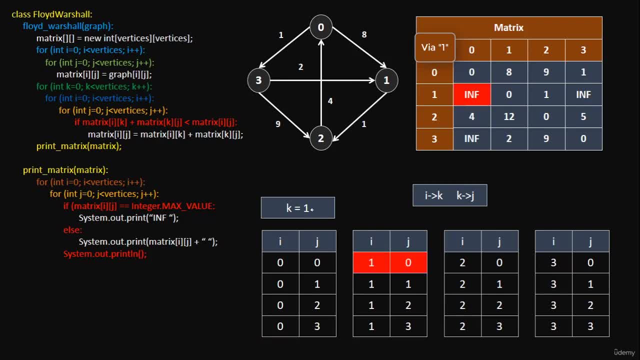 update this value here now. now, from one to one, one to one is zero and from one to zero is infinity, so we'll not update this value now. from one to one is zero, one to one is zero, so we'll not update this value. here we have: one to one is zero and one to two is one, and for this value let's. 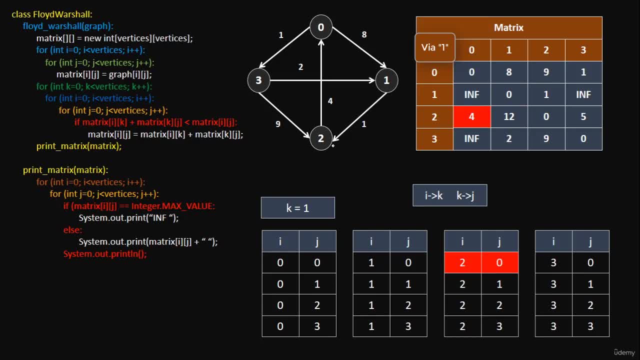 move forward. now we have here four: two to one, two to one. we see that here we have twelve and from one to zero, from one to zero, infinity, so we'll not update this value. now we have here twelve, from two to one. from two to one is twelve and from one to one is. 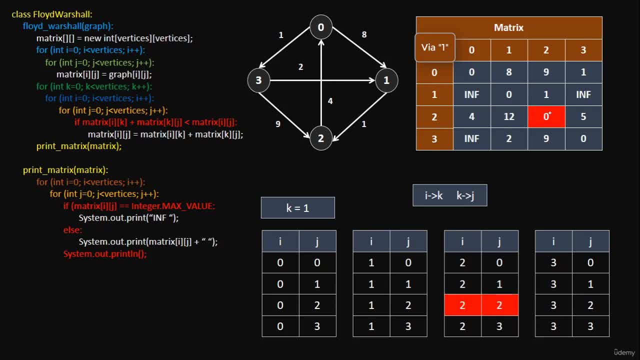 zero, so we'll not update this value now for zero. this is diagonal, so we'll not find out the value here. this is diagonal, so we'll not have any value here that less than zero. now for five. two to one, two to one is twelve. we see twelve is greater than five, so nothing need to be compared here. 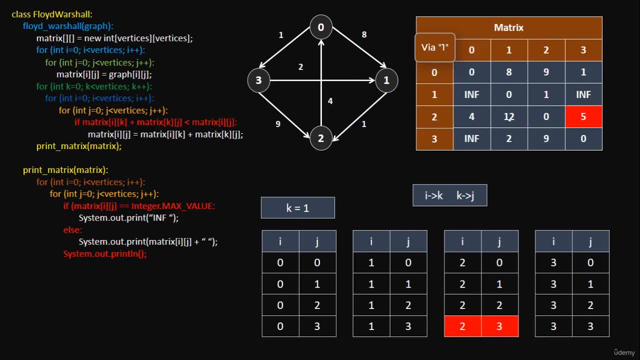 now we have two and one. now from two, one we see for two, one we have two. twelve is greater than five. now for infinity we see three to one. three to one is two and one to zero. one to zero is infinity, so we'll not change this value now for two. three to one is two, so we'll not change this value now from three to one. 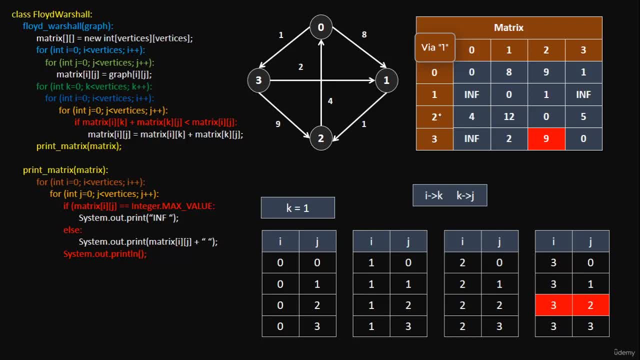 we see: from three to one is two and from one to two. from one to two is one. three to one is two. two plus one to two. one to two is one. two plus one is three. so let's update this value: nine with three. let's move forward. this is diagonal value, so there is no value that less than zero. now let's move to. 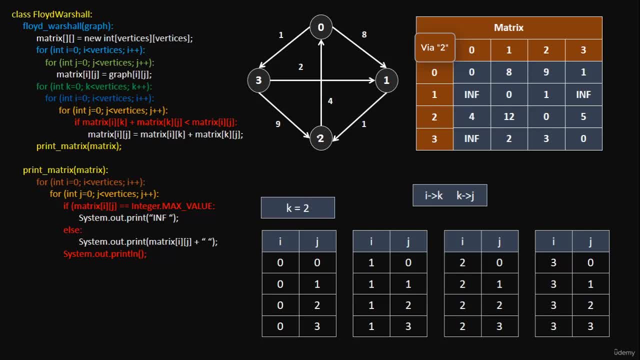 the vertex two. for vertex two, we have to find out a path from this source. that means from i to z, that that go via two, from zero to zero. we have zero here, so nothing need to be done here now. from zero to two. from zero to two is nine. we have here value eight. let's move forward now. zero to two, zero to 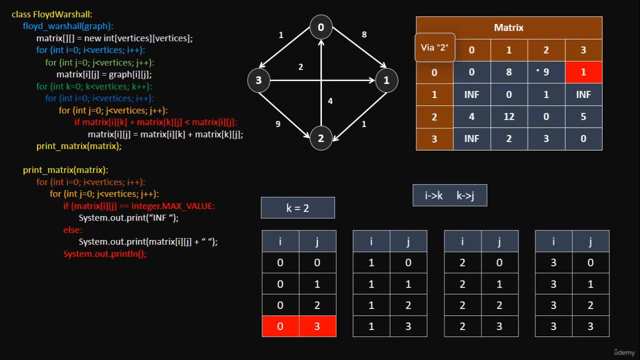 two is nine, so we will not update zero to two. the value is nine, so we'll not update this now. from one to two, from one to two, we see we have value one, one plus two to zero, two to zero five, so one plus four is five. here we see that we can visit this vertex zero from this vertex one via two. who is? 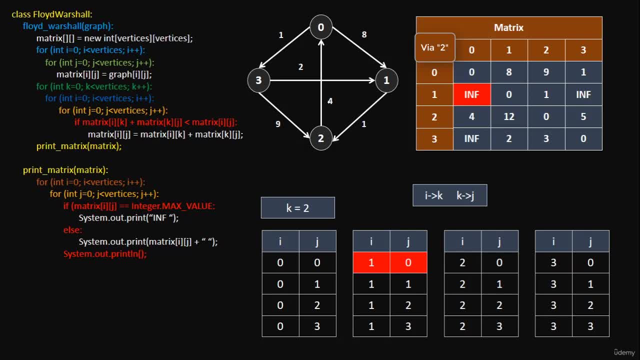 having the minimum distance here. okay, one plus four is five. so let's update this value with five. let's move forward. we have here zero. nothing need to be done here now. we have here one. one to two, now from one to two. we see that for one to two we have value here one, so nothing need to be done. 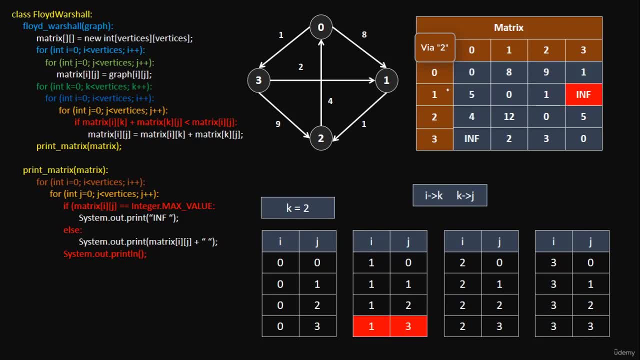 here now for this cell. one to two value: one. one plus two to three. two to three is five. one plus five is six. so let's update this value with six. we see that from one to three we can visit from one to three via this path. one plus four plus one, that is six and we have here six. hope you've understood. 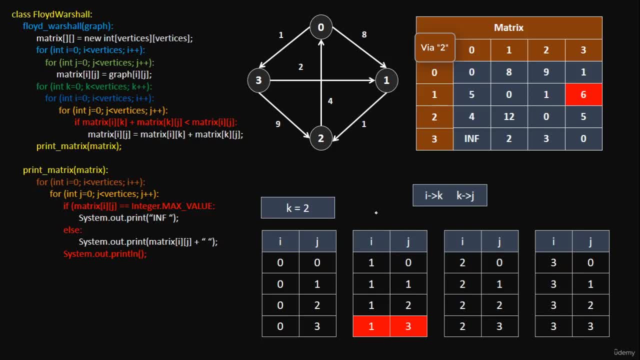 how this actually works. let me go through these examples till the end. now let's move forward here. we have four, from two to zero. we see we have a path that goes via two, so let's update this. well, with four, we see that, from two to two, from two to two is zero, zero. 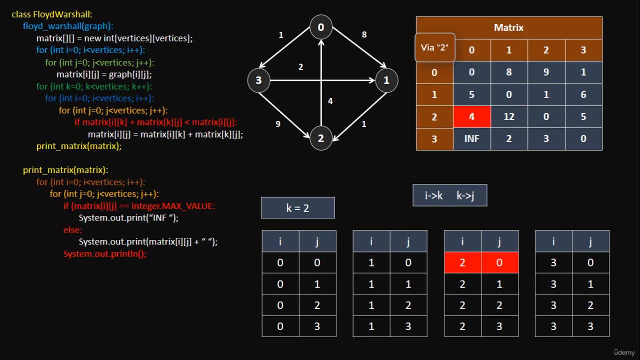 plus two to zero. two to zero is four, so nothing need to be done here. now. from two to two is zero. plus two to one. two to one is 12. nothing need to be done here. and same for the rest. and same for the rest for this row, okay. 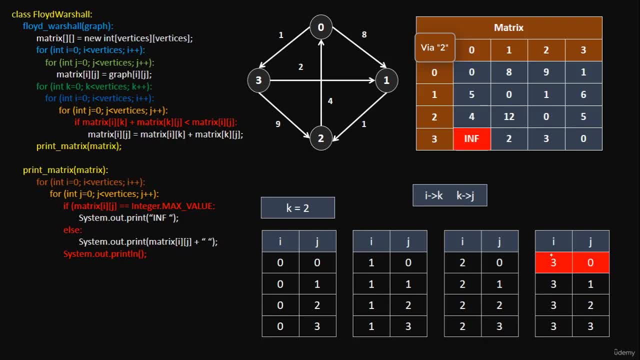 now let's move forward here. we have infinity. we have 3: 0 from 3 to 2. from 3 to 2, we have 3, 3 plus 2 to 0. 2 to 0 is 4. 3 plus 4 is 7. let's update this value with 7. okay, from 3 to 0, we. 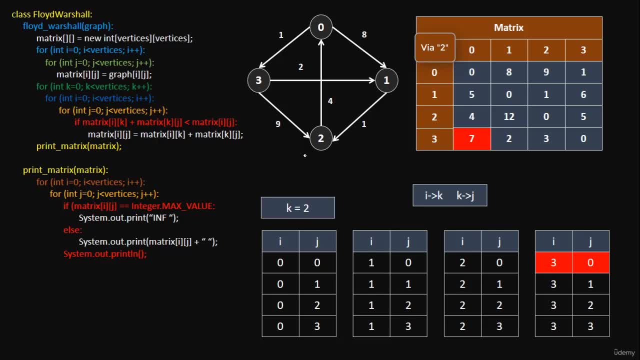 see we can go from 3 to 0 in this path. we see that we can go from 3 to 0 via 2 in this path: 3 to 1, 1 to 2, 2 to 0. okay, and this is the summation of the path distance. okay, 2, 1, 4, that is 7 we have. 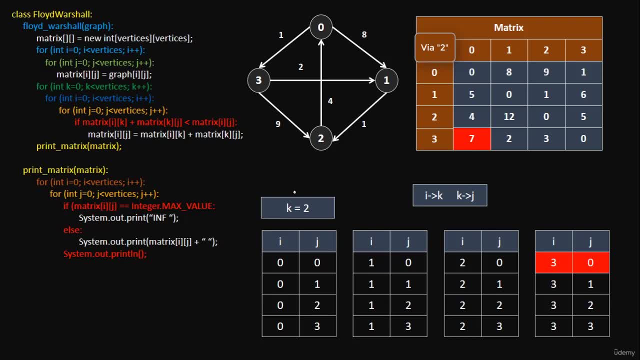 already calculated for 0 and 1. now we're calculating for 2. okay, we're using pre calculated result to generate this value 7. so this is a dynamic programming. try to relate this with the previous result of dynamic programming table. this is a little bit intuitive now. let's move forward now from 3 to 1 via 2. 3 to 2. 3 to 2. 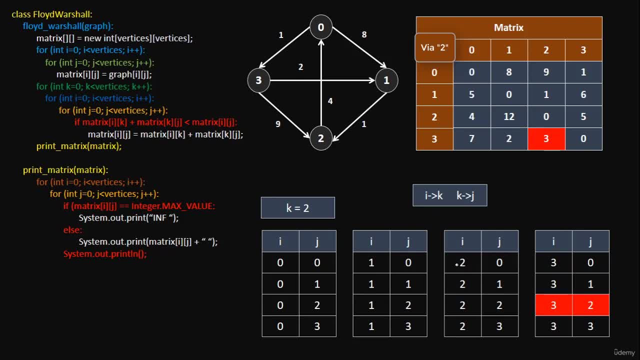 is 3. 3 is greater than 2. let's move forward now from 3 to 2, that is 3. 3 to 2. 3 to 2, that is 3. let's move forward now from 3 to 2, that is 3. 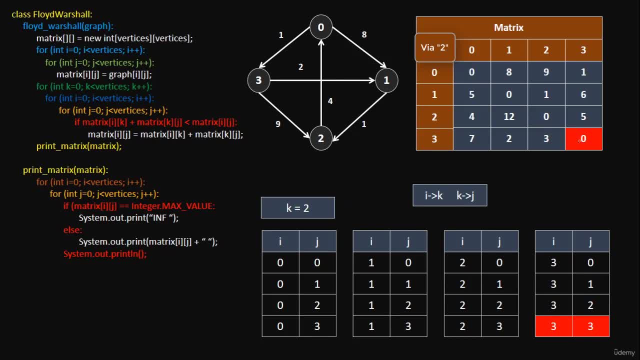 now from 3 to 2, that is 3, 3 to 2. 3 to 2, that is 3, 3 to 2. 3 to 2, that is, It will be 5, 4, 4, 4, 4, and this product will make it to a, isn't a. 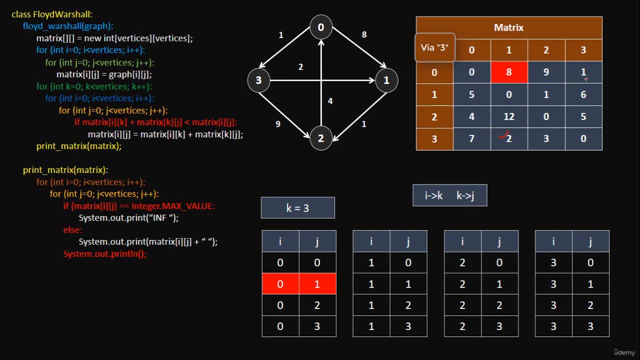 zero. so 2 plus 1 equals to 3. let's update this value with 3, because 3 is less than 8. let's move forward: 0 to 3, there is 1 and 3 to 2. 3 to 2, that is 3. 1 plus 3 is 4. let's update this value with 4. 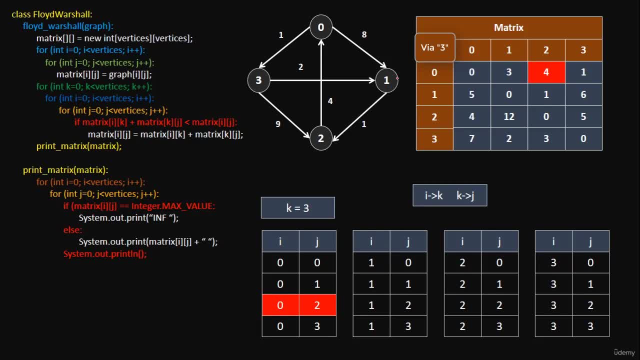 and here we see that from 0 to 2, from 0 to 2, that goes via 3, the path is 1 plus 2 plus 1, that is 4. let's move forward: 0 to 3, that is 1, so we'll not change it now. 1 to 0. 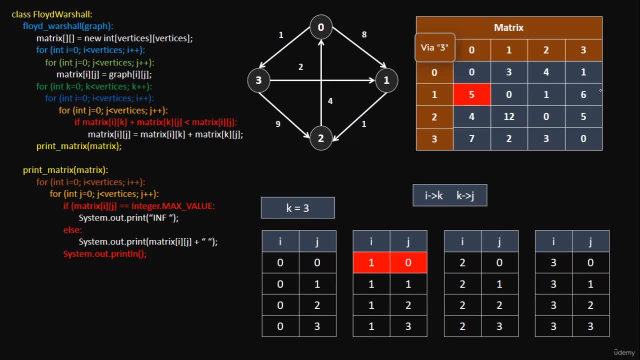 here. from 1 to 3, from 1 to 3 is 6. 6 is greater than 5. let's move forward. here again, 6 is greater than 0. let's move forward, let's move forward. let's move forward now for this value. 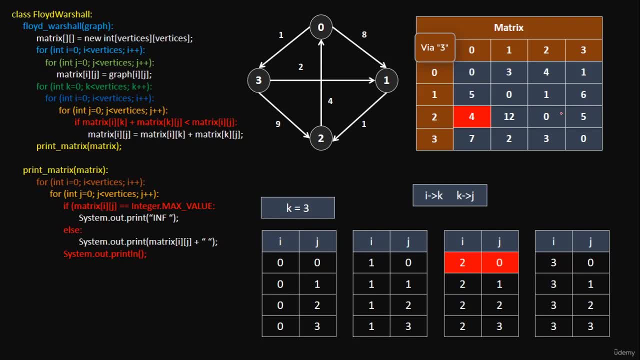 okay, 2 to 3. 2 to 3 is 5. 5 is greater than 4. let's move forward now: 2 to 3: 5. 5 plus 3 to 1. 3 to 1, 2, 5 plus 3: 7. let's update this value with 7. let's move forward. it's 0, so it will not changed. 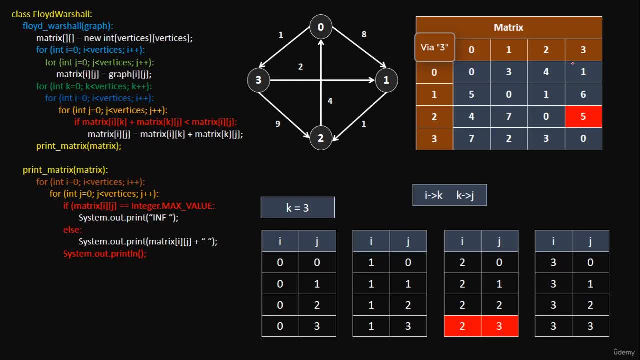 let's move forward 5: 2 to 3: 5, so we'll not change it. let's move forward 7: 3, 2, 3, 2 to 3. there is 0, 0 plus 3 to 0. 3 to 0 is 7. 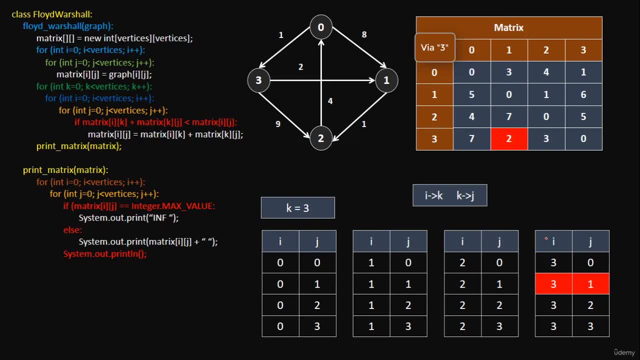 0. 3 to 0 is 7, so you will not change it. 3 to 3: 0. 3 to 1 is this value, so we will not change. for the rest, we're done. we find out this, we find out this matrix, okay, and this matrix contains: 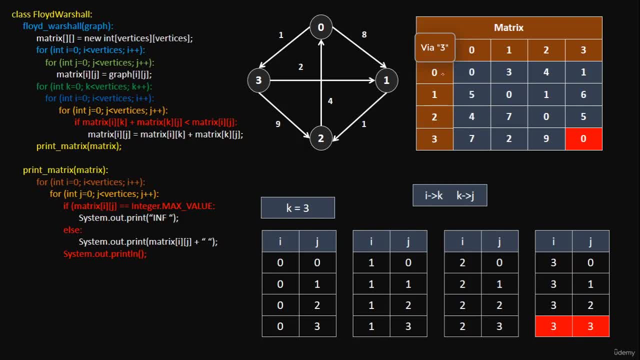 the minimum means of minimum distance from the vertex 0 to all other vertex, from vertex 1 to all other vertex, from vertex 2 to all other vertex and from vertex 3 to all other vertex. this is called floyd virtual algorithms. we are generating all possible pair that might go through k and we're calculating. 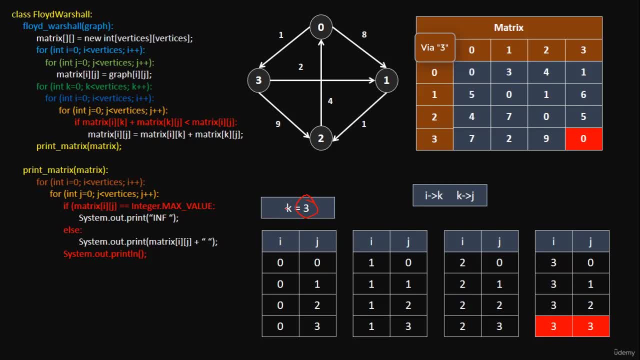 the minimum path, and this is called the floyd algorithm, since we're generating all pair for all vertex. so we'll have the minimum path. this solution will takes big of nq time complexity and this solution will takes big of n square space complexity to create this matrix. okay, 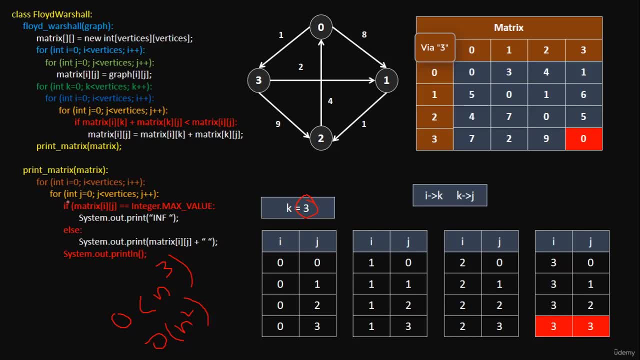 and here we're printing this matrix using this function: print matrix. hope you've understood how floyd version virtual algorithm works. if you have any question, if you have any suggestion, let us know. if you have any question understanding this video explanation, post your question on the q and. 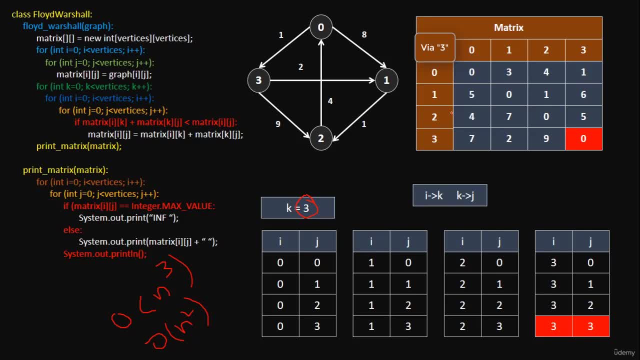 a forum. i'll be glad to help. thanks for watching this video. i will see you in the next video. 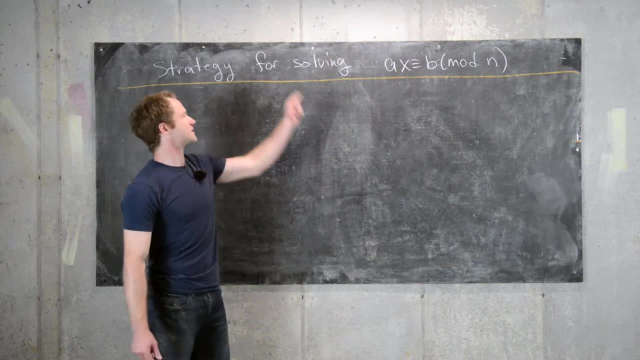 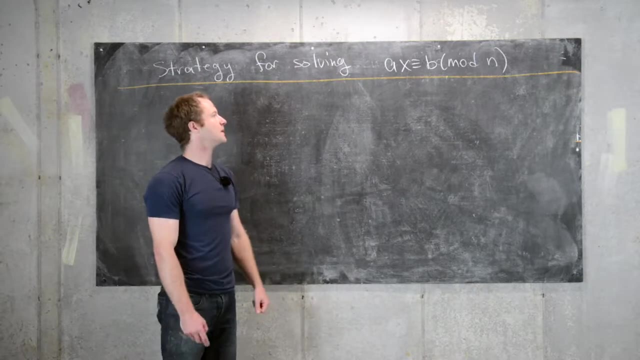 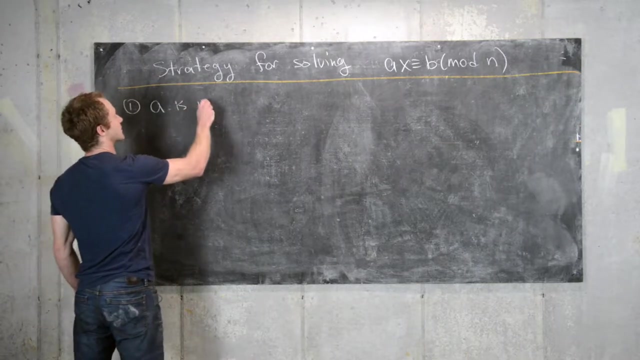 Okay, so in this video we're going to outline a strategy for solving linear congruences. AX is congruent to B mod N, and then we'll look at an example. Okay, good, So maybe the first part of the strategy is to notice that A is invertible. 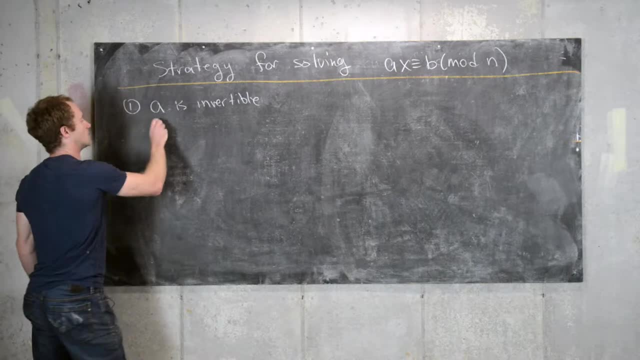 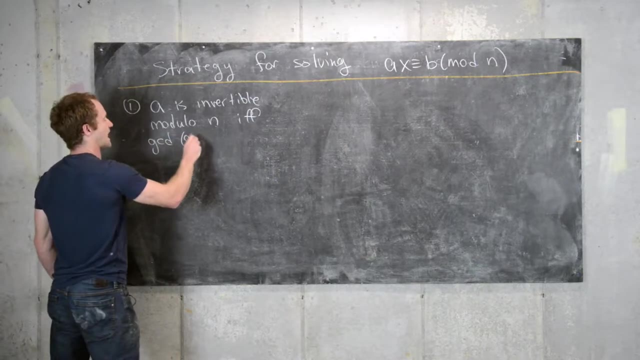 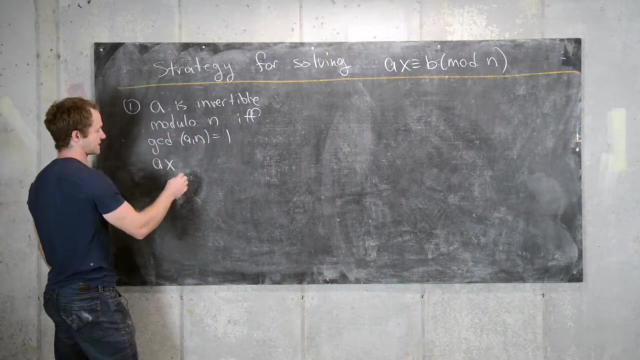 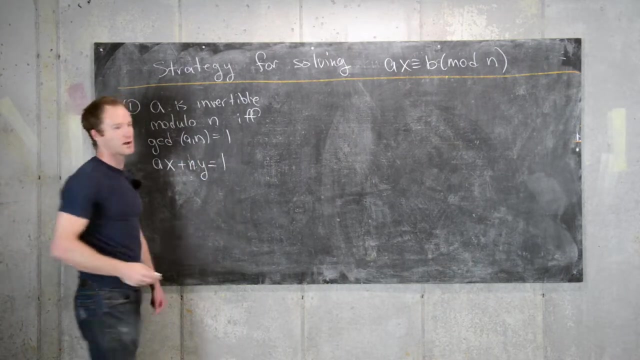 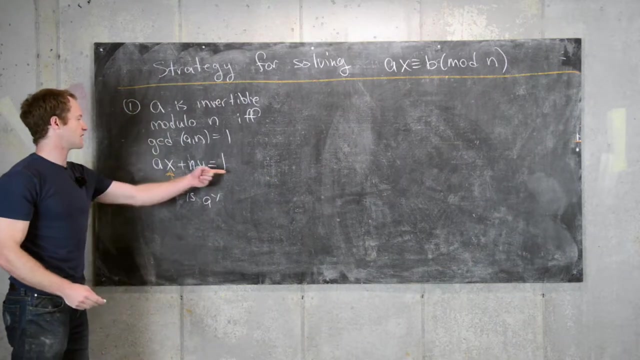 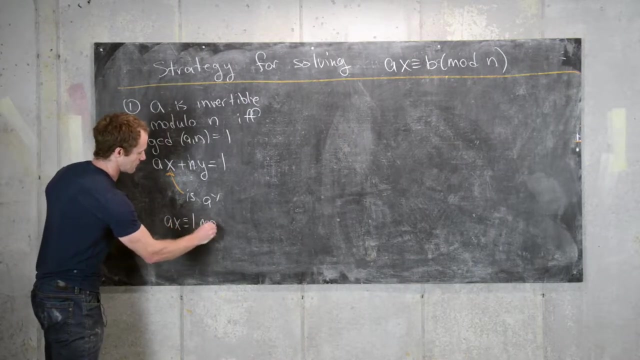 modulo N, if, and only if, the GCD of A and N equals 1.. Good, And in that case you can solve AX plus BY- sorry, plus NY equals 1, and this value of X is A invertible Inverse, Because if you look at this equation, modulo N you have, AX is congruent to 1 mod.